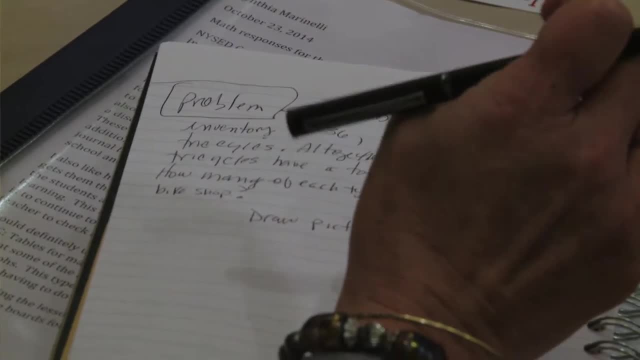 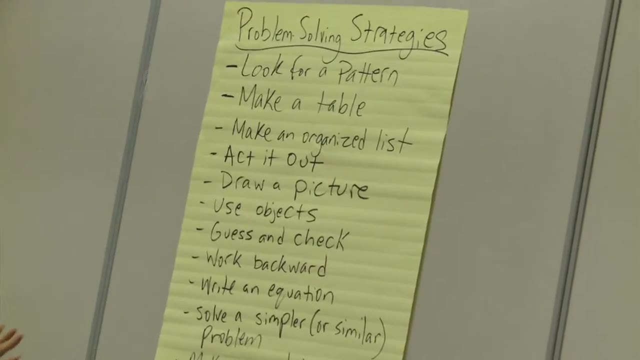 of them are tricycles, And before they do any work, I ask them to read the problem and then look over the list and then write down any strategies they think might help For the problem. solving strategies: which ones do you think? which ones stood out to? 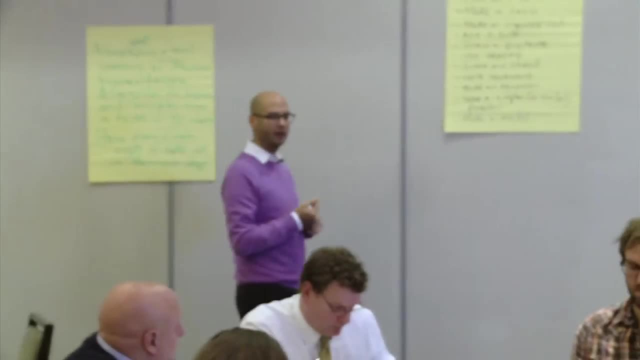 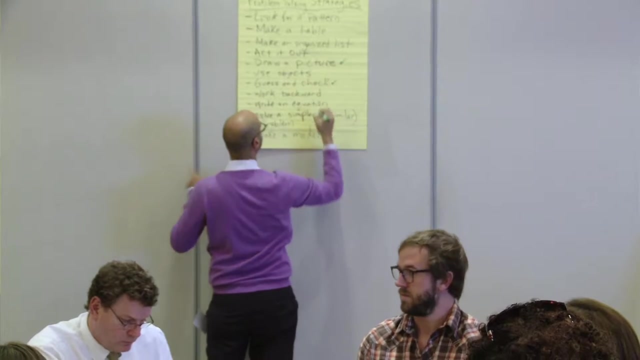 you. maybe that might be a way I could approach this problem. Just call them out and I just want to kind of make a notation of guess and check, Okay, Picture Objects. And the reason why I do that is because we need to help them develop an awareness, be conscious of when. 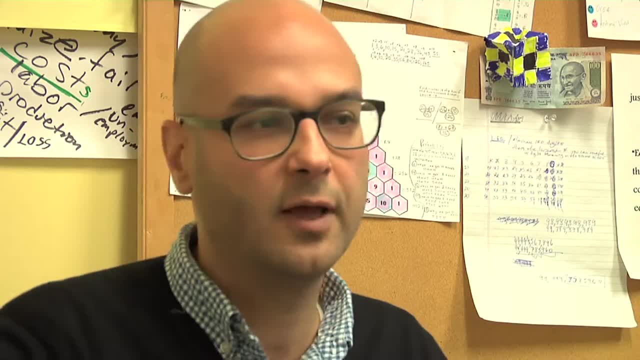 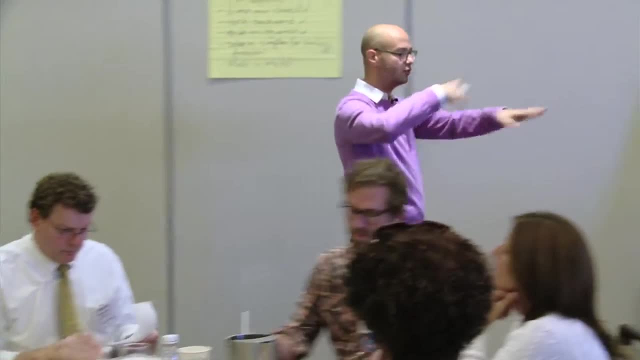 does it help to you know when I'm drawing a picture? When does making a chart help? Which of those strategies helps me when I get stuck? So now share your tables. You can work in pairs or in your, in your whole table. 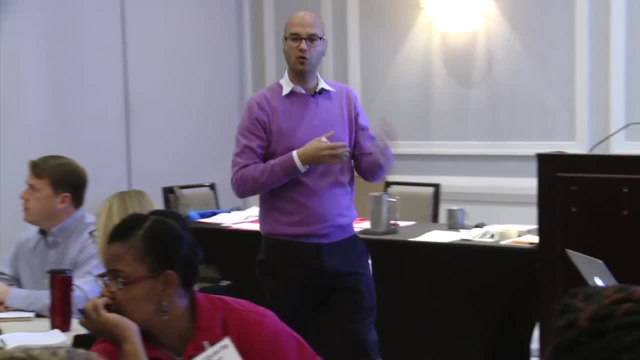 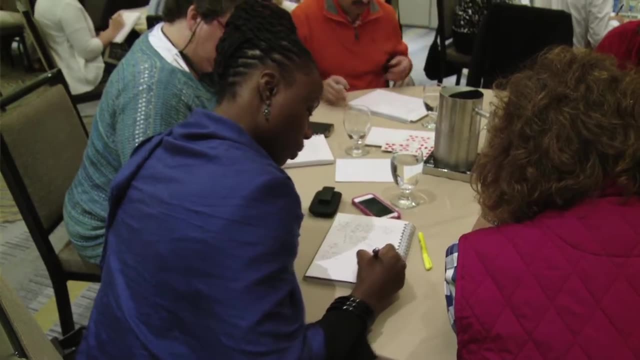 Now implement those, try them out, see which ones work, see which ones don't work. So then I let them work and I let them struggle. I don't tell them how to solve that problem. I give them that problem and give them the strategies, and then they're messing around. 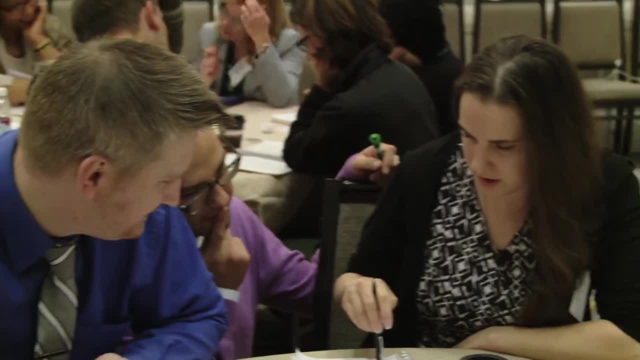 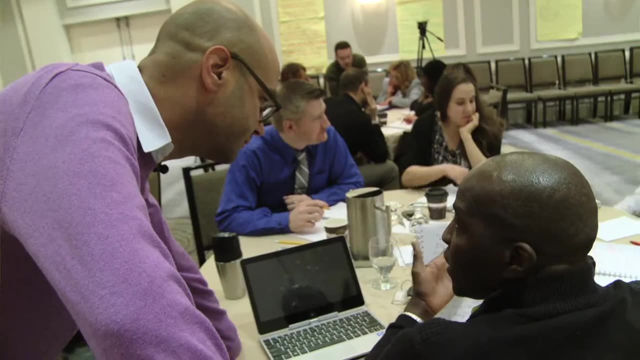 with it, And so, as I'm walking around, there are a couple of different things that I'm doing. One: I'm trying to help people who are stuck, But the other thing that I'm walking around doing is what are the problem solving strategies that I want to highlight For the 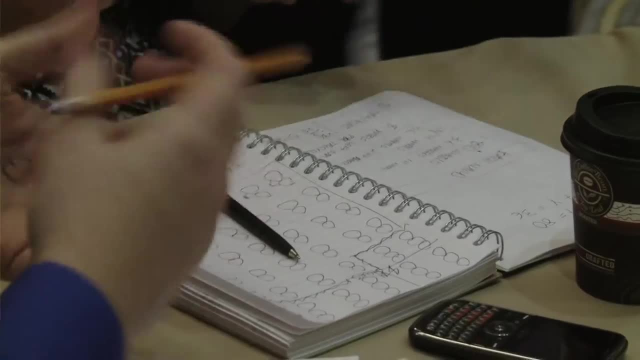 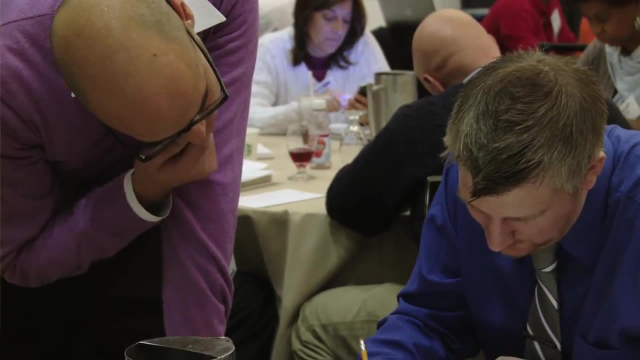 bicycle shop problem. the three problem solving strategies are drawing a picture, guess and check and making an organized list or chart. Students are working. What I'm doing is I'm walking around the classroom and I'm looking for someone who's got a picture. I'm looking for someone who's using guess and check And 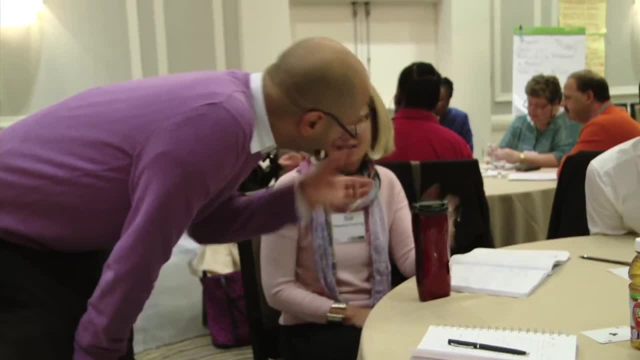 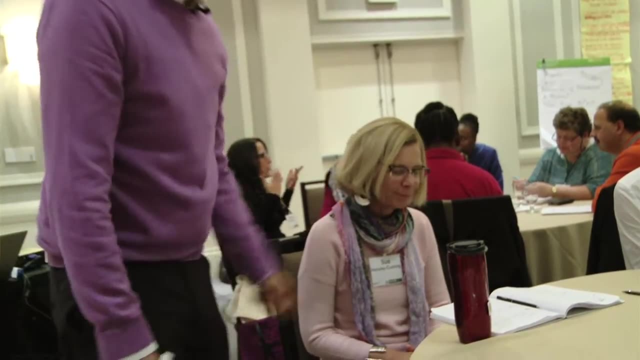 I'm looking for someone who's making a chart. Oh, I'm sorry you didn't right, Because it's guess and check, but you did guess and check in an organized way using the table. And if I don't see any of those strategies, I'm going to be looking for stuck students. 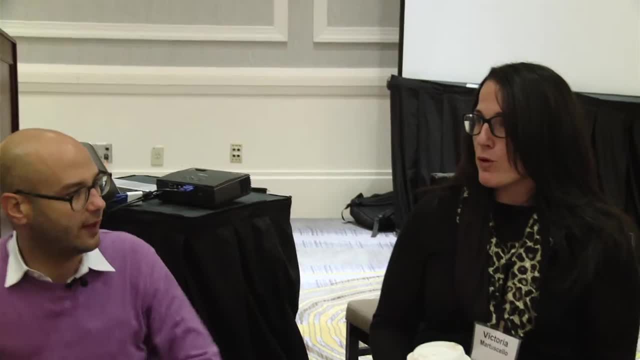 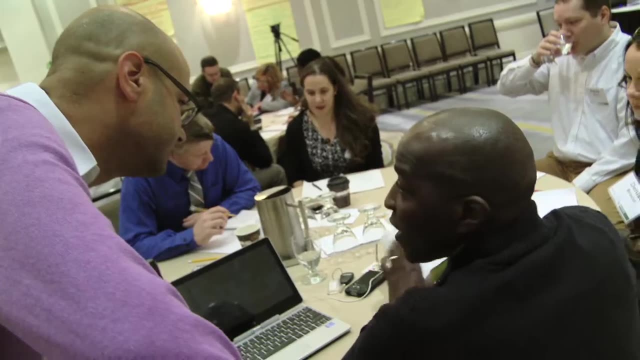 and I'm going to be saying: can you draw a picture of the situation or a visual representation of the situation, just so that we can kind of make sense of it? And if I'm looking for guess and check The question, I'll ask them: well, what could it be? Can there be a hundred bicycles? And 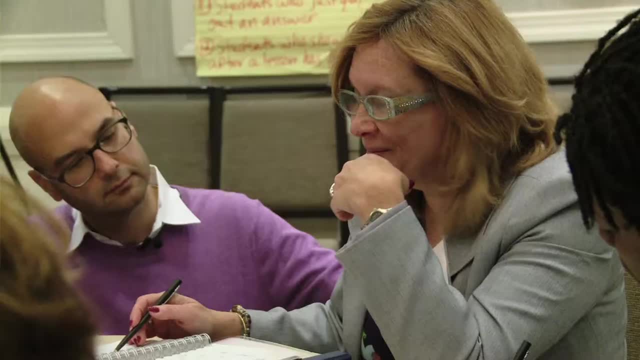 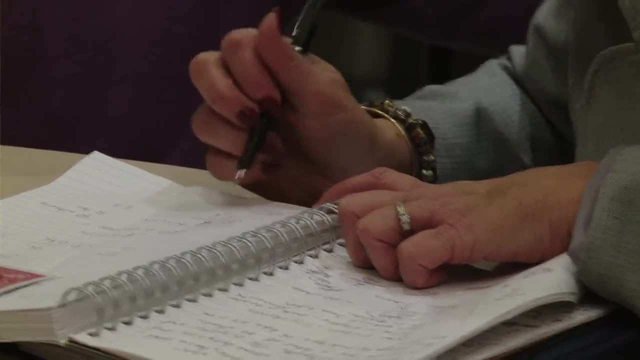 they'll say, no, Oh, why not Making a guess? but then how do you check it? And then for making an organized list or a more organized chart, I'll often ask students who have done guess and check: is there a way to organize your thinking a little bit? 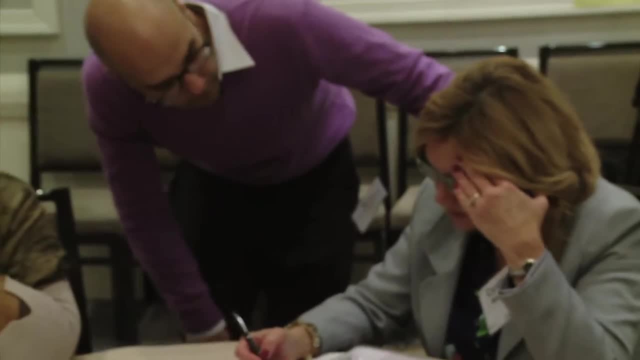 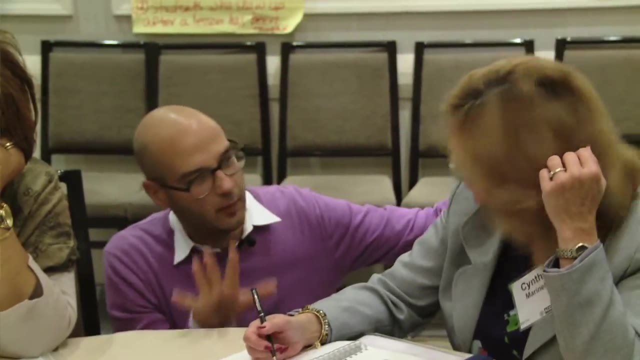 And I'm breaking. It's going to be a little bit more organized on my paper here. So, yes, And then this has to be because it has a T. So this is not one of those situations that I'm describing right now, where I'm just going to say who wants to come up and share. 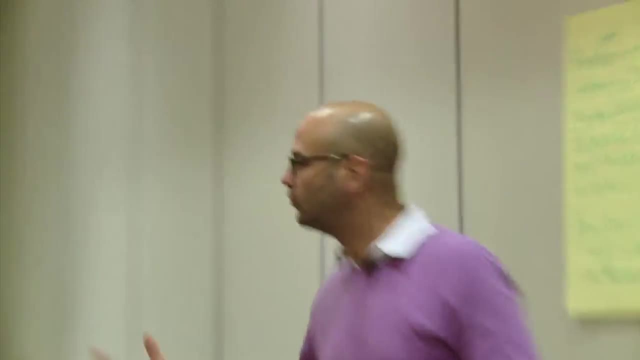 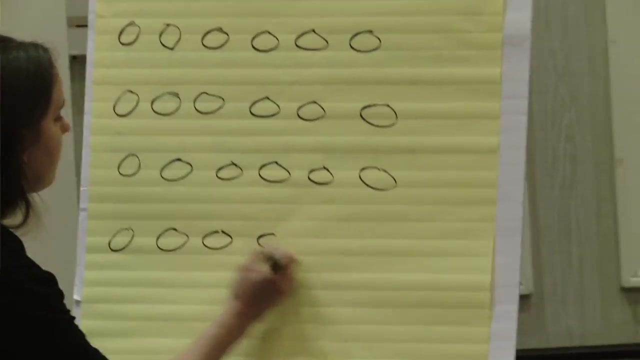 their answer, Because I have specific things that I want to show. So what we're going to do is we're going to look at a couple of different strategies that people have used to solve this problem- okay, And we're just going to talk about it, And not only do I. 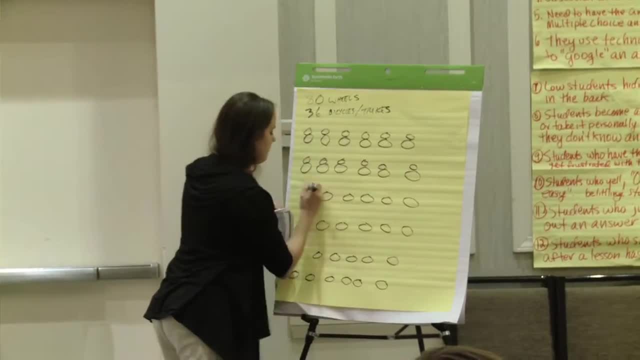 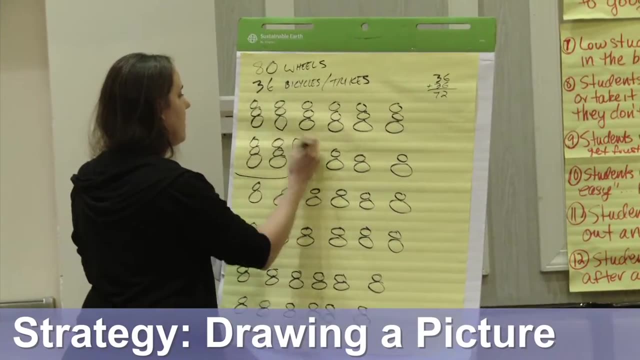 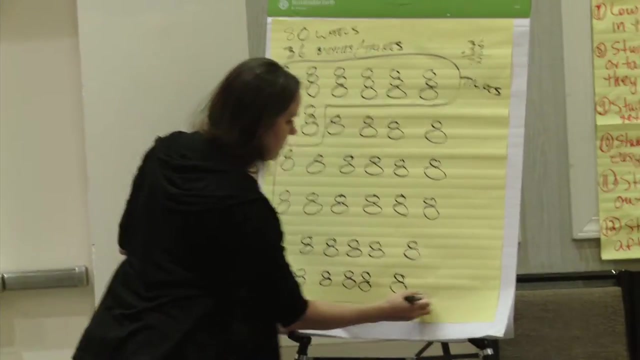 have specific things, but I have a specific order in which I want them to go up. I'm always going to have the visual one, the picture, go up first. That's one that everybody can see. So 980.. So these guys are my tracks, And these guys are my tracks, And these guys are. 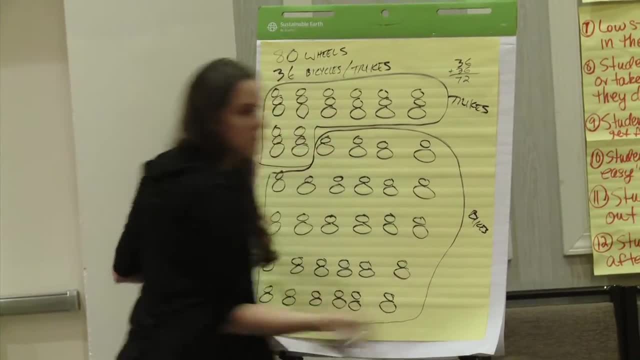 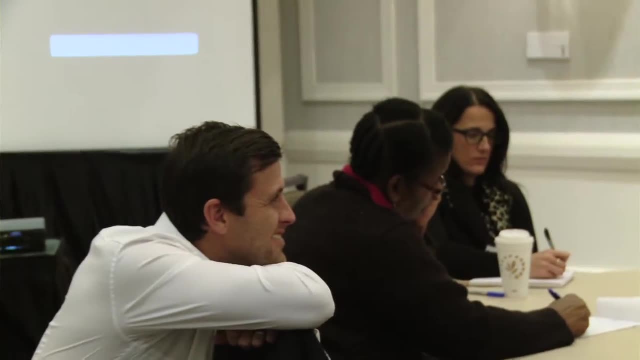 my bikes Pictures can be very elegant. When the picture goes up, there's almost always this like: that is really cool and interesting And I didn't even think about it that way. And that happens both when teachers are doing this problem and when students are doing the problem. 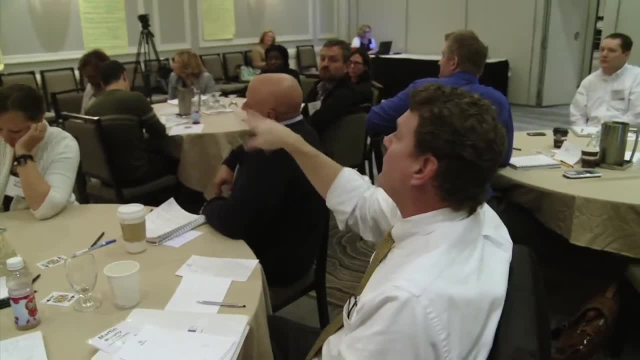 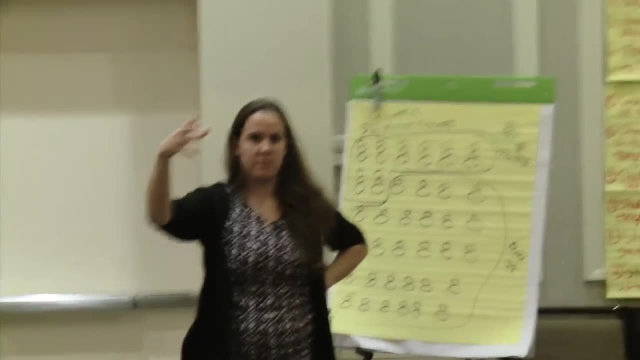 Real simple. I missed the beginning, when you decided how many bicycles you were going to start with. Well, because the problem said that there were 36 bikes and trucks together And we had 80 wheels. So I knew, I knew. 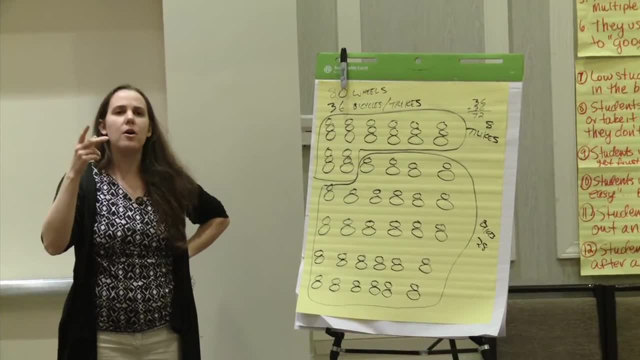 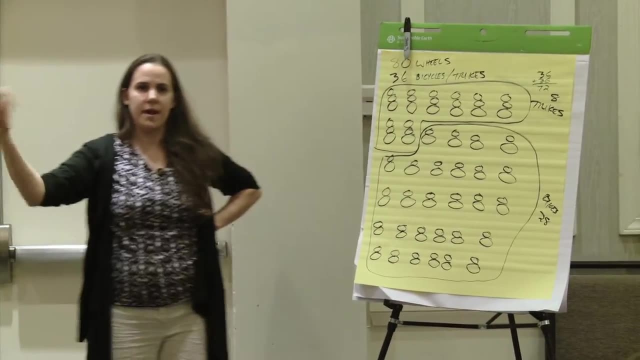 I knew 36.. Everything's going to get one wheel. And then, oh, there's no unicycle, so everything's going to get two wheels. And then I got to keep adding wheels to the extras until I run out of wheels. 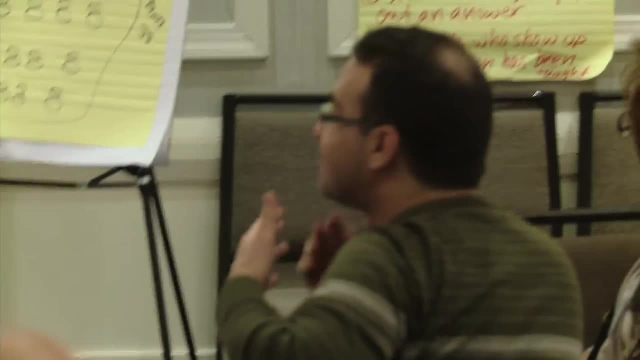 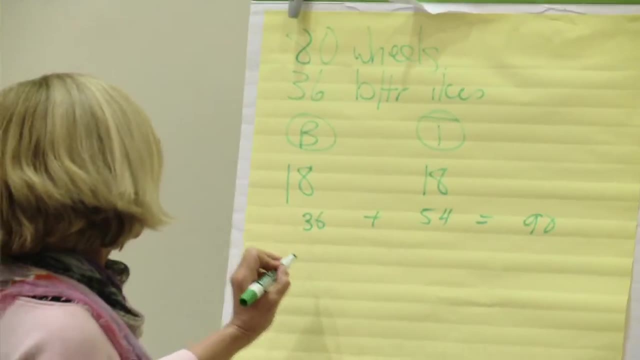 Gotcha. As Aaliyah said, it's so visual and also so easy. It's just- it makes sense, Guess and check. A lot of things happen with guess and check. I want students to understand that it's actually a strategy. 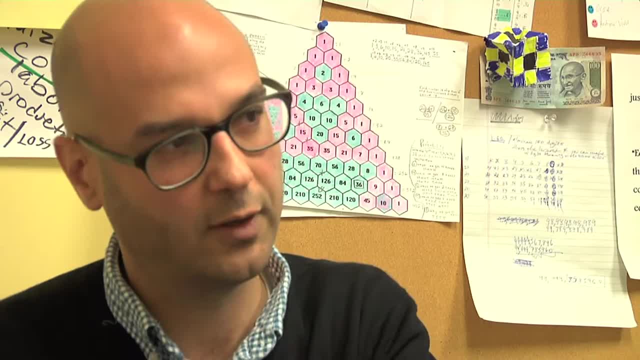 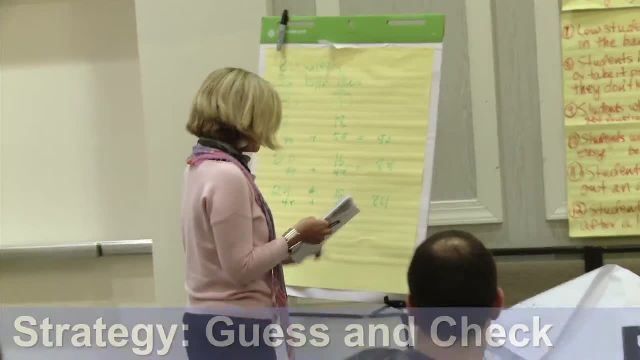 There's a lot to learn about how to do it. They're using the guesses that don't work to make their next guess: 48 plus 36,, 84. So we're definitely going in the right direction. Now I got overconfident. 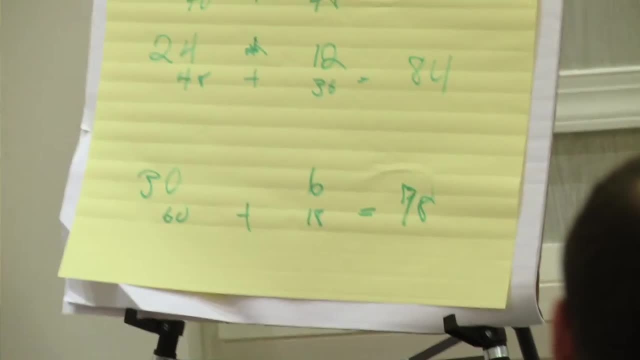 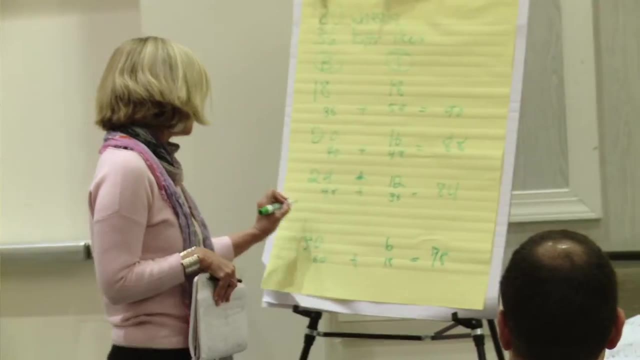 So I went right to 30.. That's a really important process that takes practice. The students have to see it, but then they also have to start actually practicing how to do that, how to use the guesses and checks that don't work. 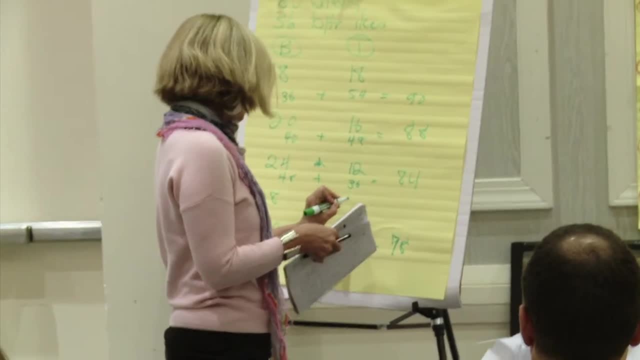 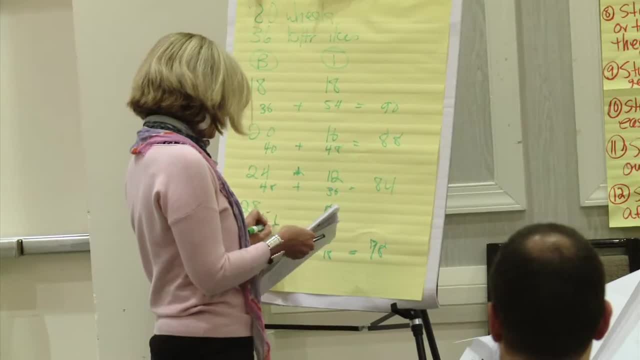 And then I'm going to go to the next guess, And then I'm going to go to the next guess, And then I'm going to go to the next guess. So now we're on 54.. 56 plus 24, equaling goal-wide 80.. 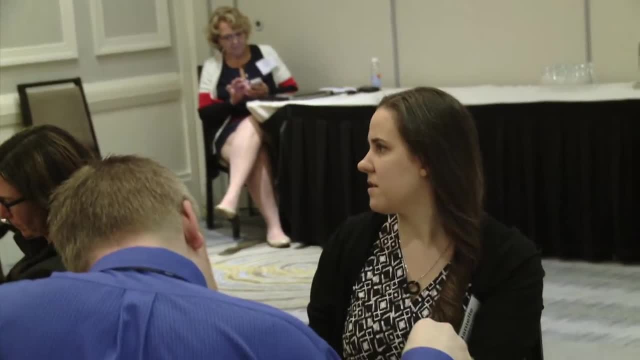 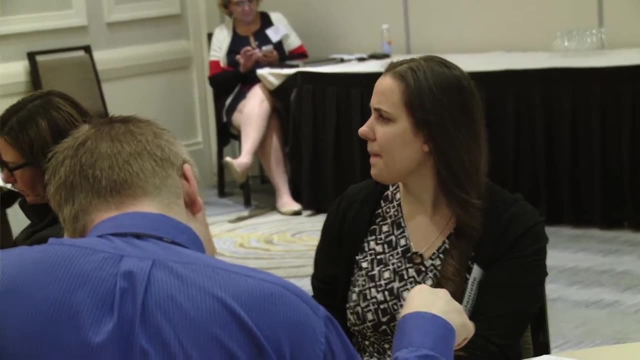 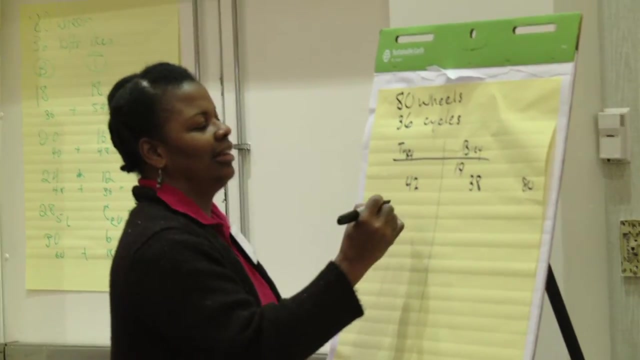 Your way allows you to see the pattern of what's happening in a way that the drawing one didn't quite make it as apparent. Two things happen when students look at the organized chart. One, they start seeing that that you can be more thoughtful in the way you're guessing and checking. But the other 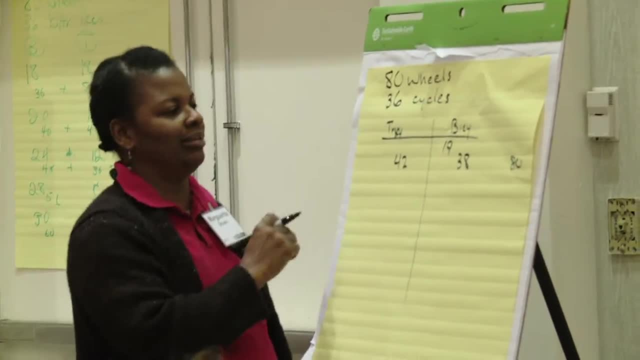 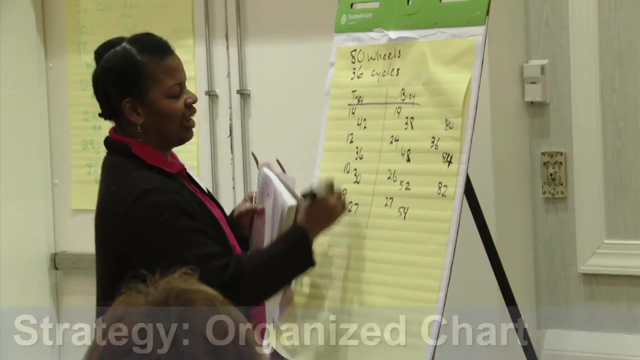 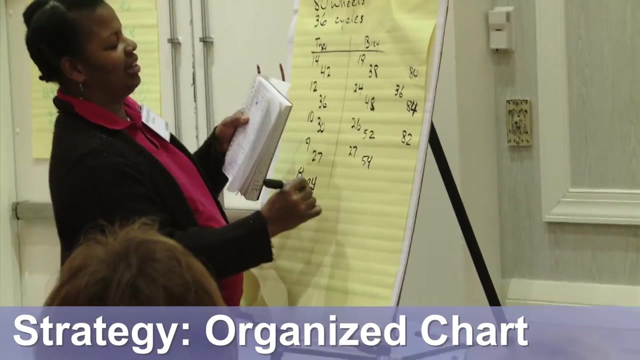 thing that often comes out in conversations is that because you can say, oh, every time I remove a bicycle, this happens to the wheel, the wheels. When you have all of the numbers there, you can see pattern. So I gotta go down again. So I got to eight and I did 24 wheels, Like I have a good feeling. 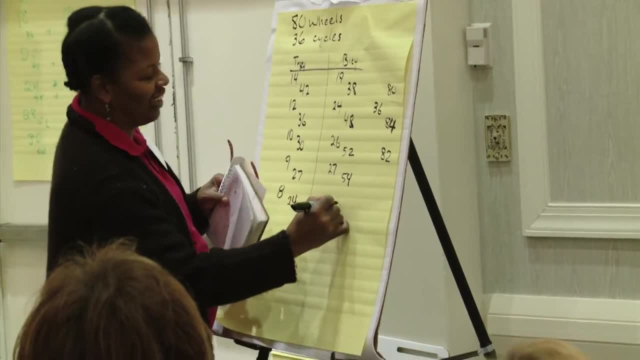 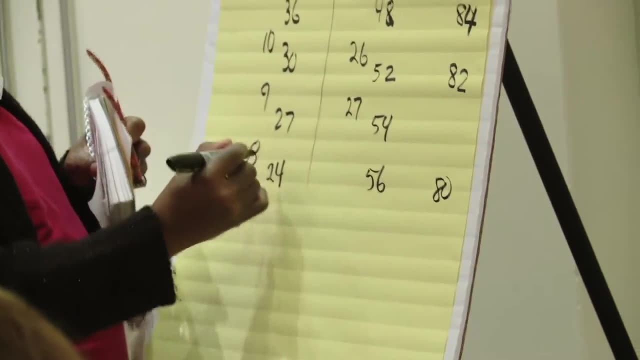 about this Drum roll, you know, and then it's like: okay, good, It's gonna work. This is 56 wheels and that's 24, and that's 80 wheels, So there are eight of those and there. 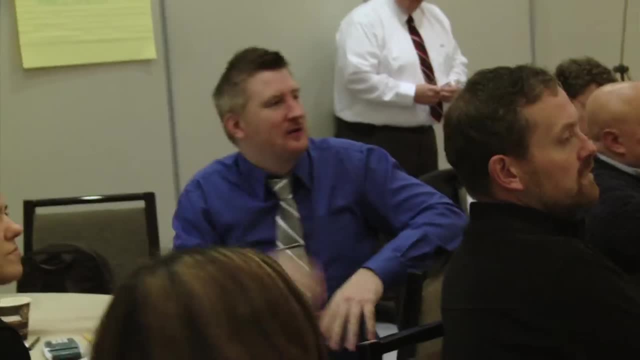 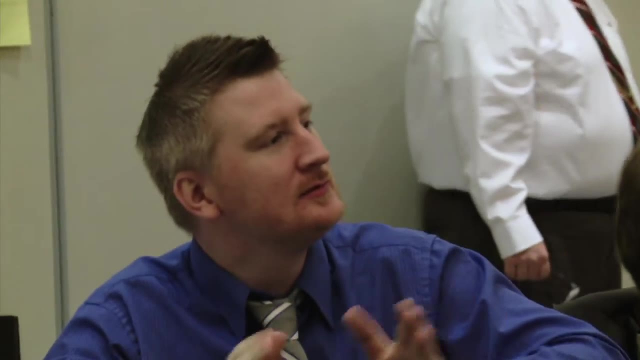 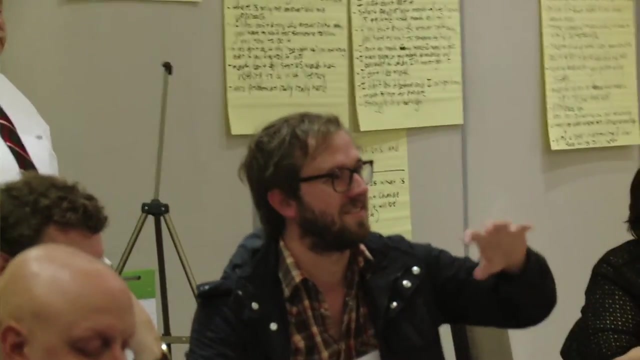 are 28 of them. I just like the organization of it. You broke down into a chart: Bicycles one side, tricycles the other side. Those three students are sharing their strategies, not only to celebrate their own work but because they allow us all to have to kind of think about those strategies that are going. 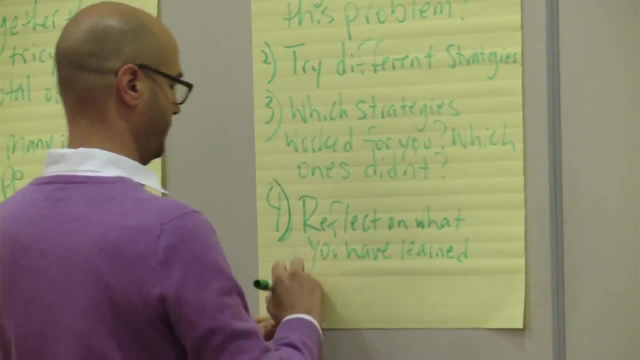 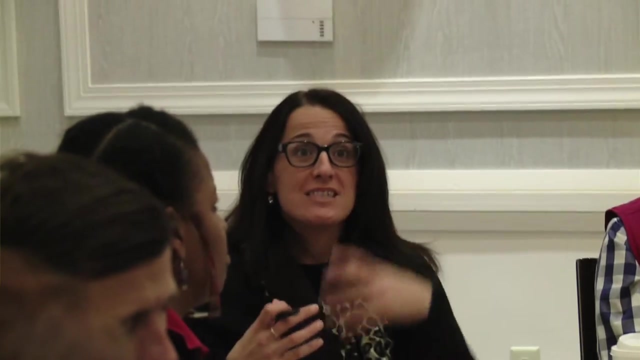 up. So then, the final thing I have students again kind of reflect on. so pick a problem-solving strategy, and what have you learned about that particular problem-solving strategy? Their big takeaway is: wow, it's, that's just great. 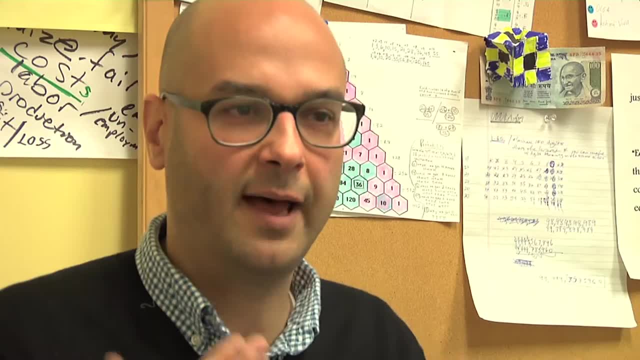 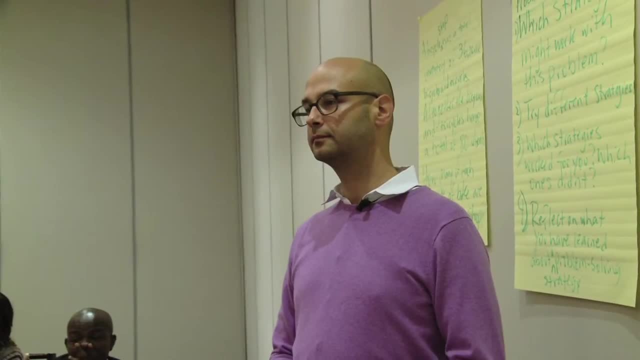 It's crazy. Those look very different. It kind of is breaking them of the mindset of there's only one way to solve it. I think it was very helpful. I really love having a list up. You know, I've done this with my class and I've done a table type of a situation, but I kind of just went straight. 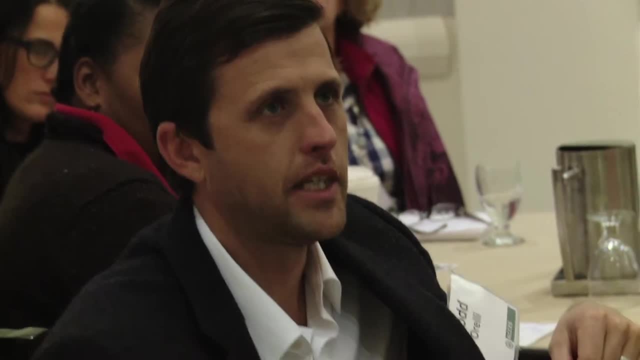 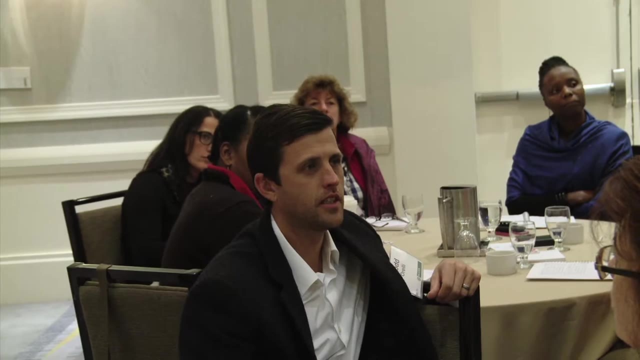 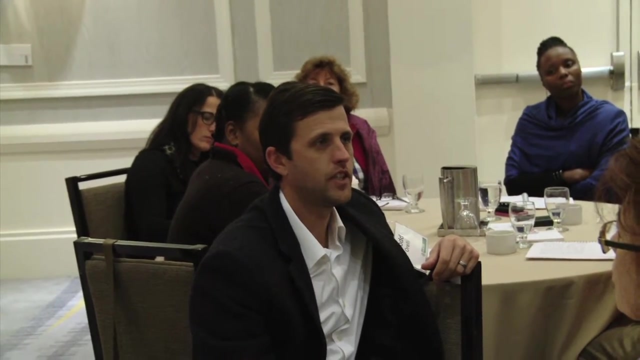 into a table and as a strategy. But I like that this is actually having them kind of develop a possible list of avenues to attack something before they get to it, which I haven't really done before. So I love just like listing all the strategies first as a good starting. 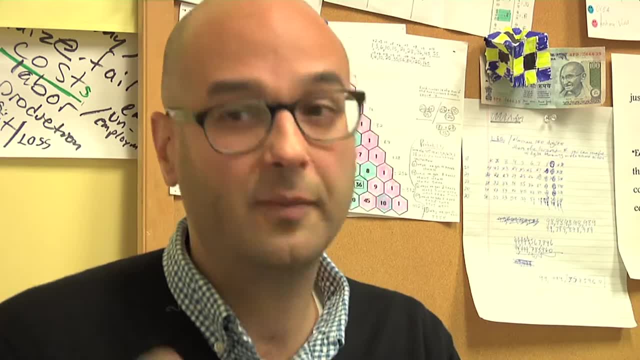 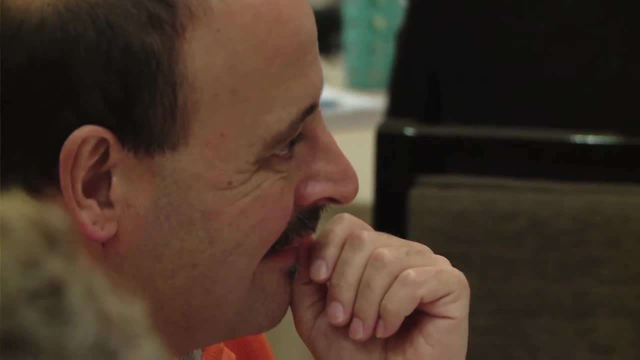 point. That's huge. That's a really important thing to do in the beginning of the semester. but then continually throughout, Kind of make them stretch and say I'm learning a general problem-solving skill. I didn't just learn how to solve this one problem. That's kind.